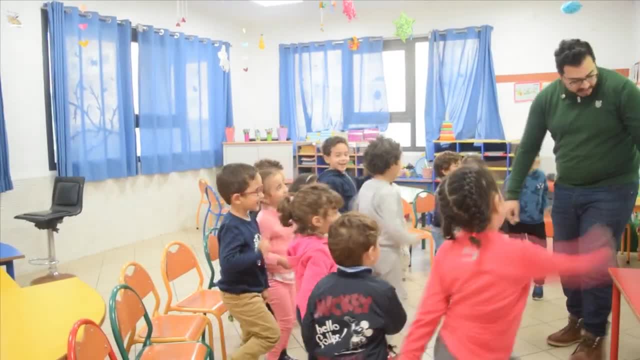 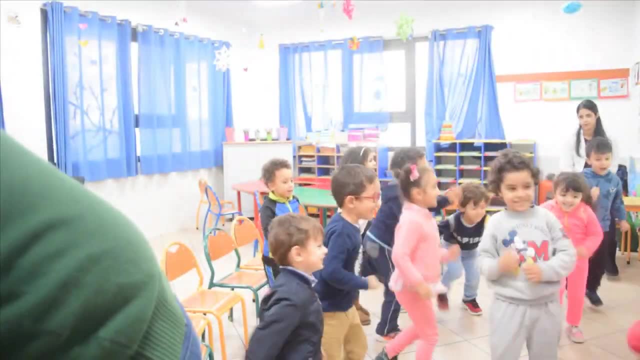 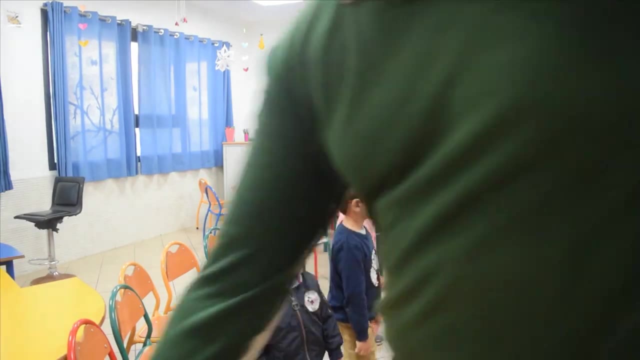 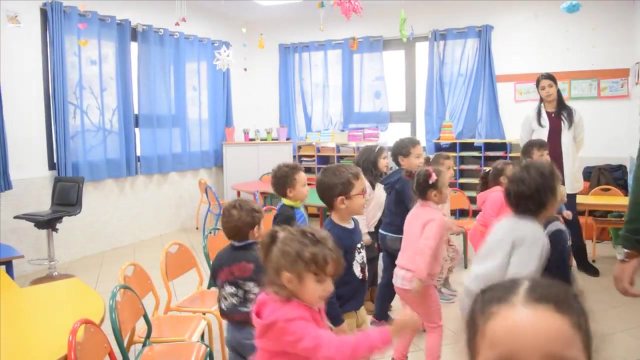 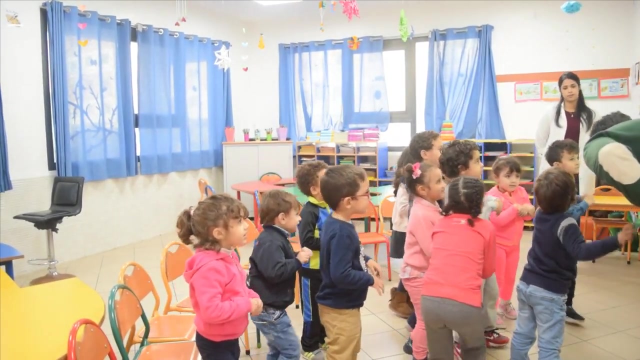 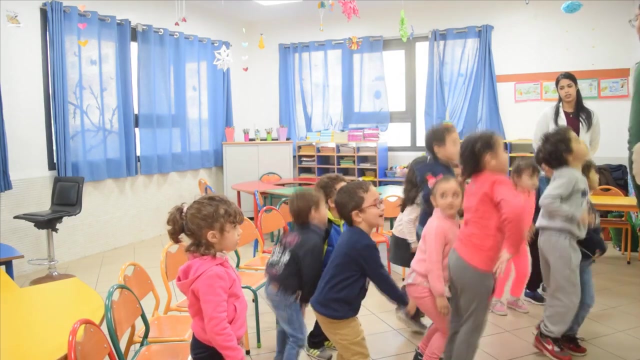 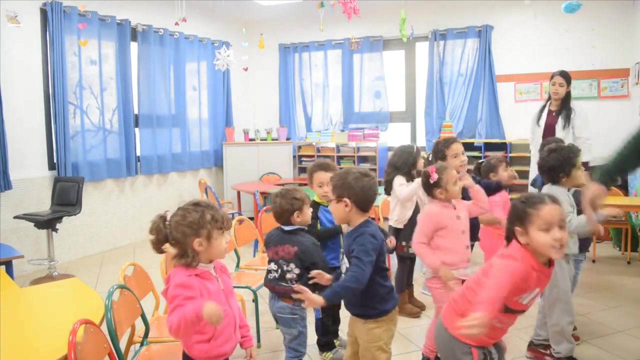 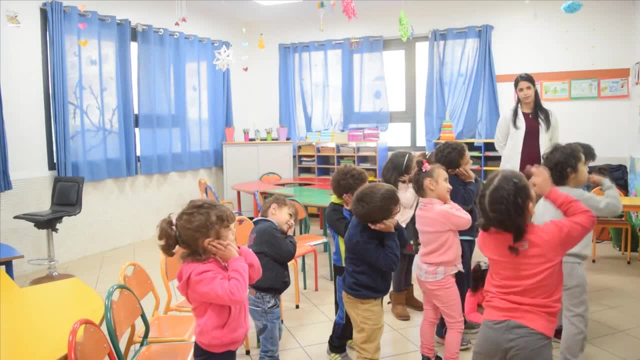 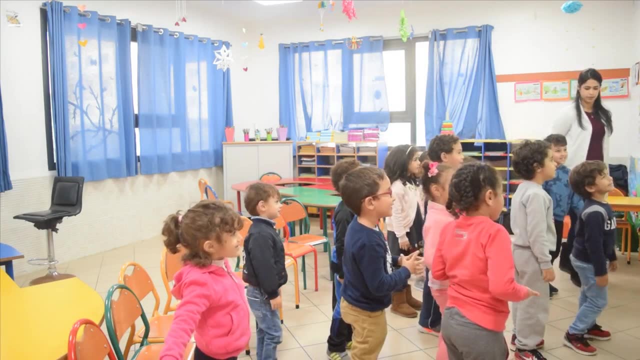 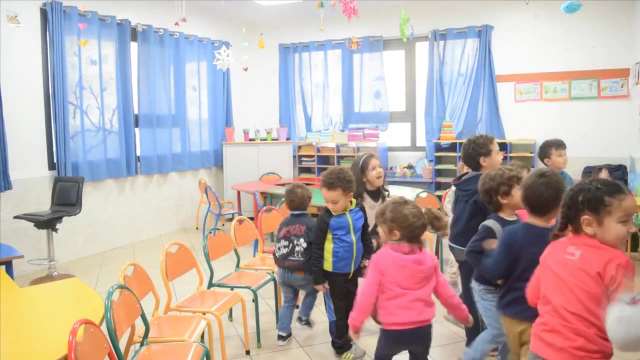 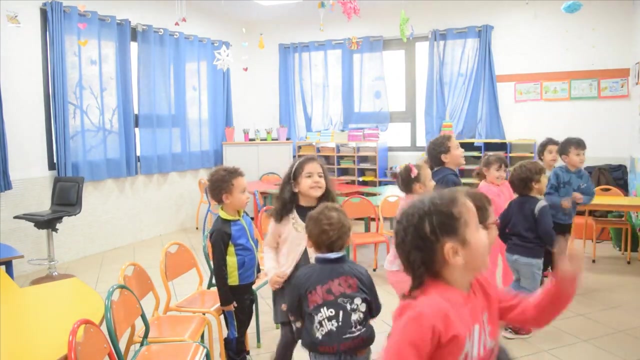 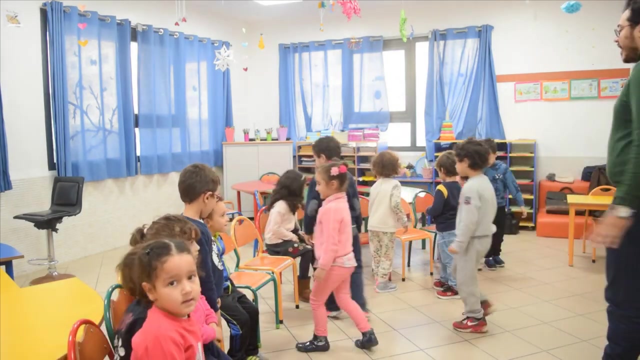 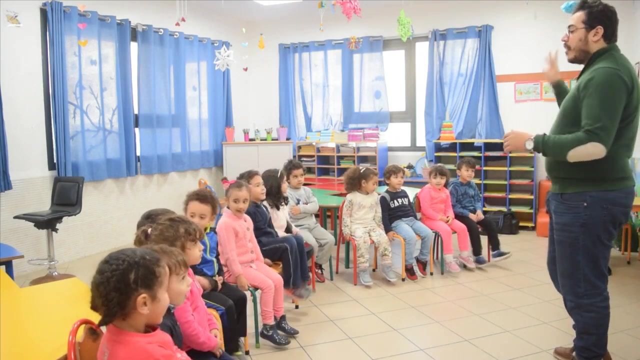 Now let's sleep. Wake up, Wake up, It's time to jump. Okay, sit down everyone. Good, Now you sit down. you sit down. That was really good. Okay, We sit down. very good Now in three: two: one: 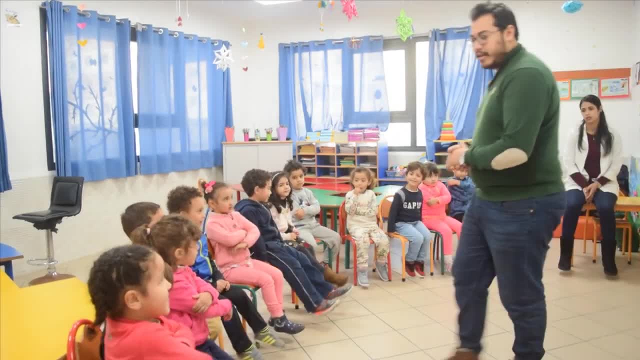 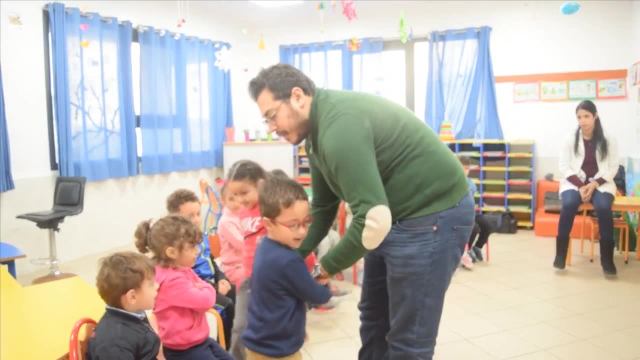 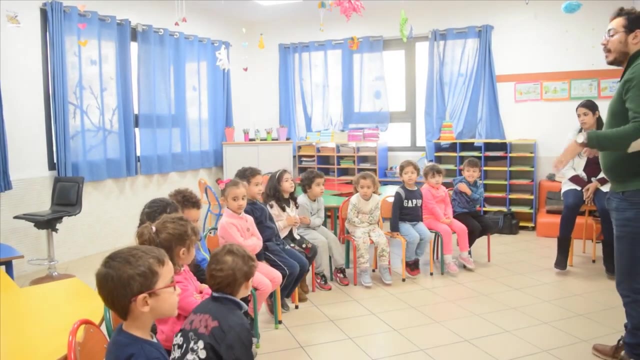 One, Let's do it. OK, Come here, Anish, We touch, We touch, And you little boy down there And I touch. Good, Now, guys, you say after me: Hey, Anish. Last time 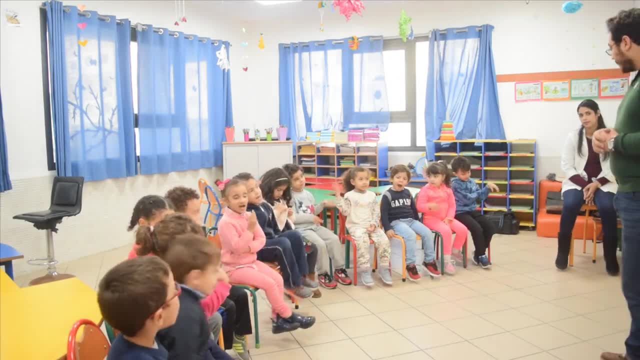 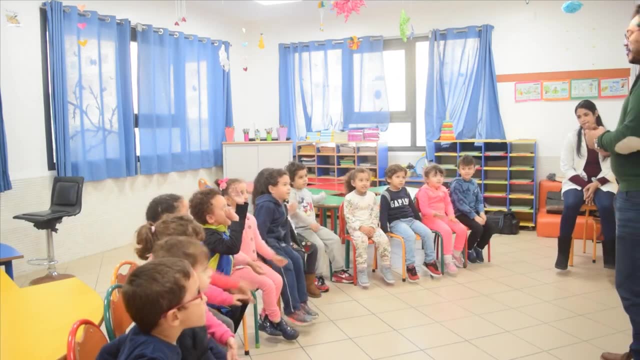 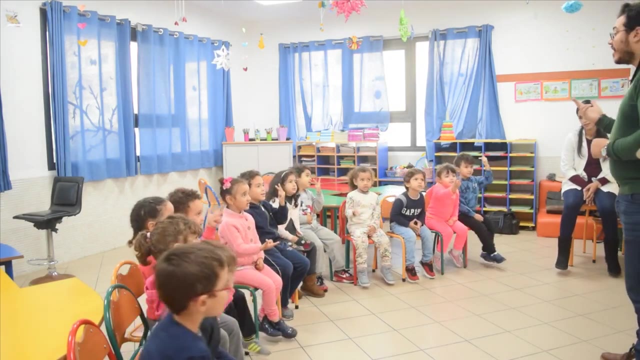 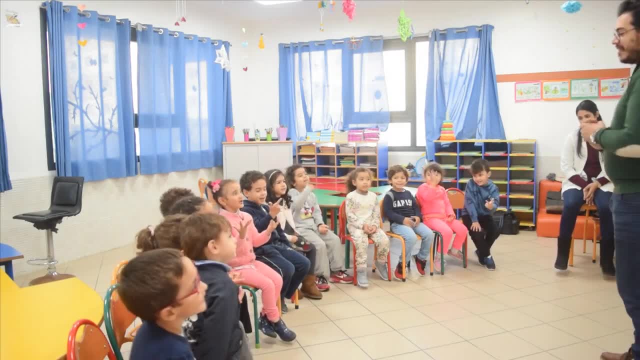 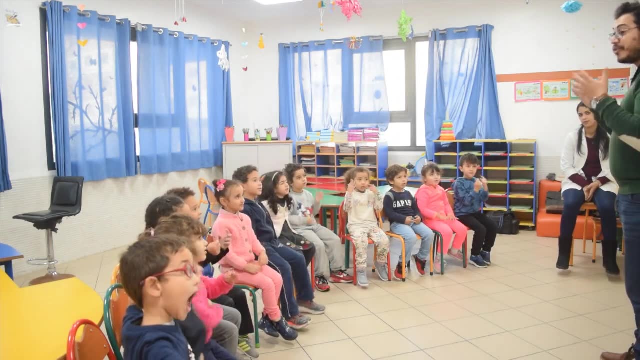 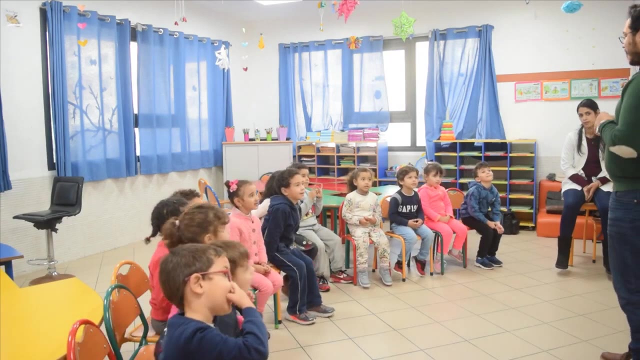 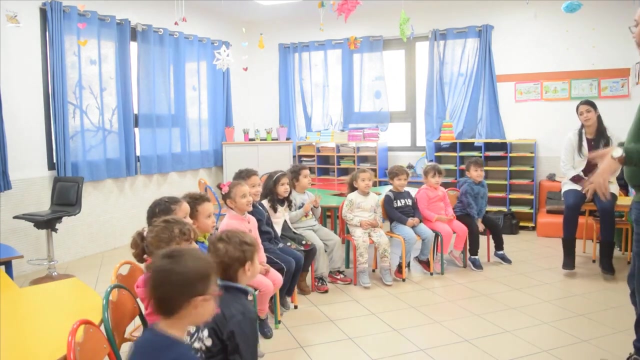 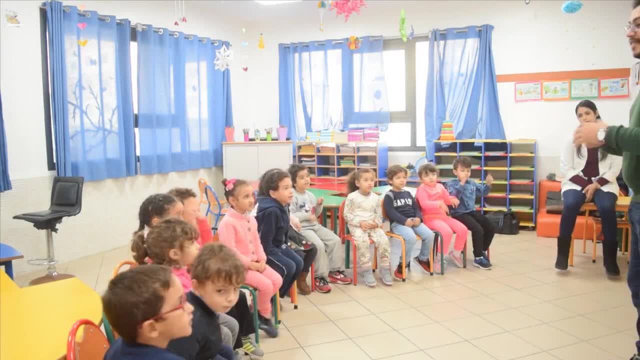 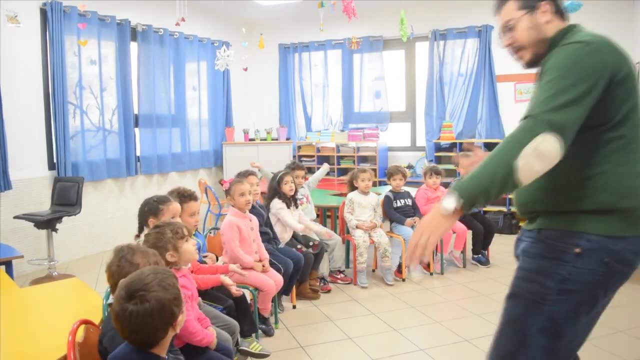 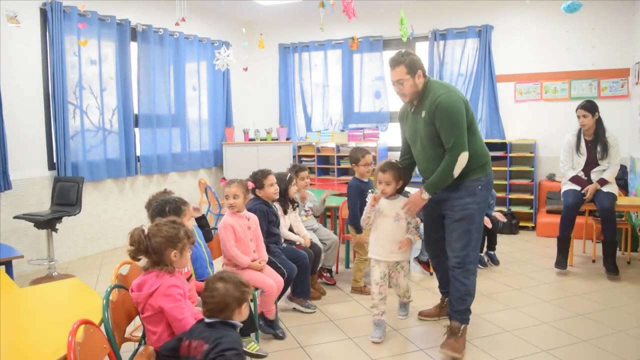 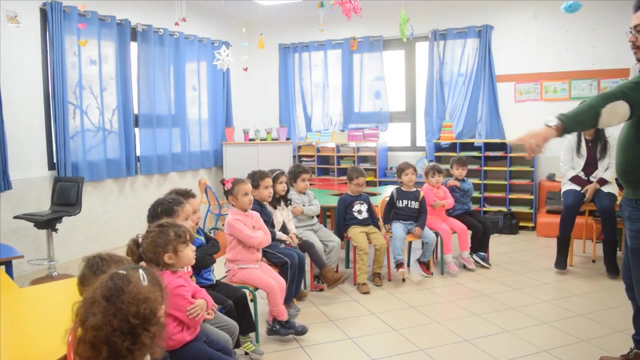 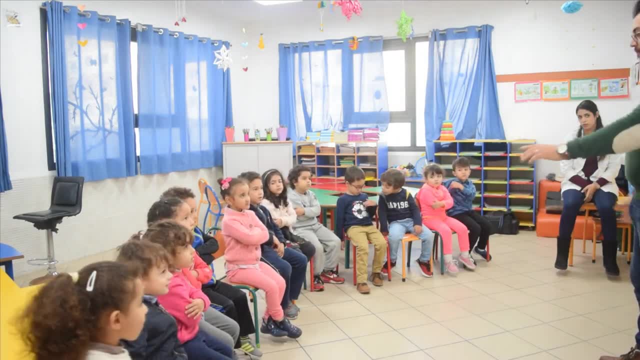 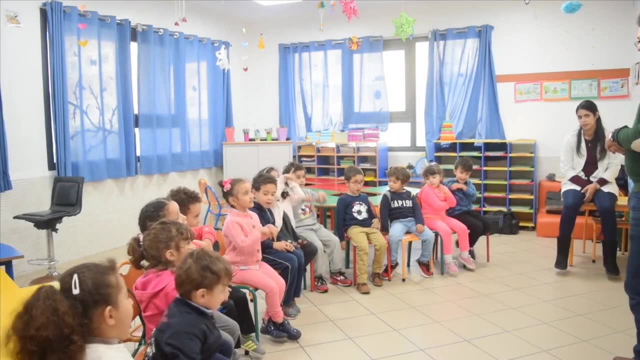 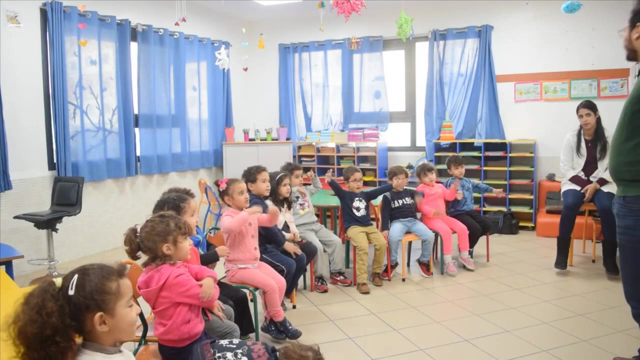 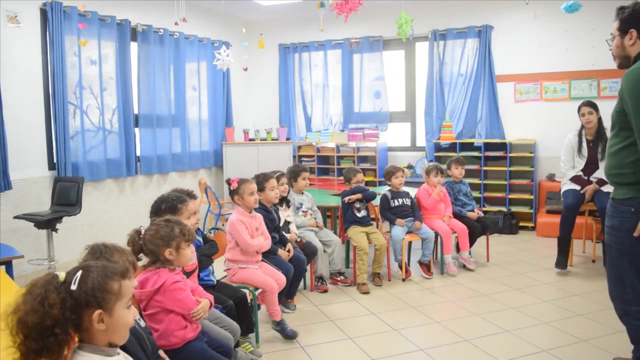 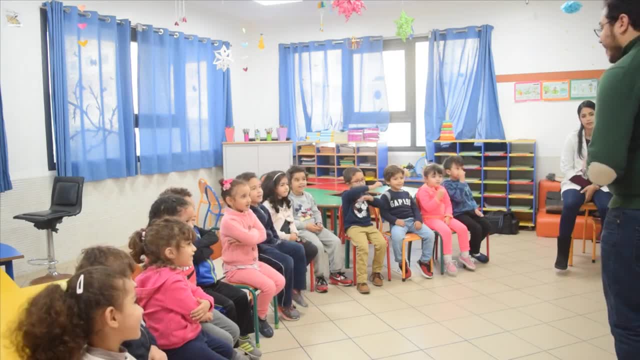 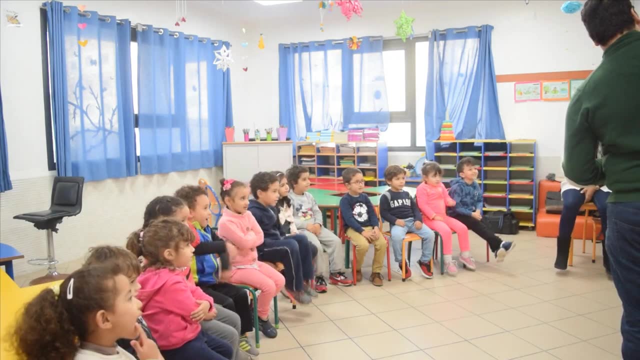 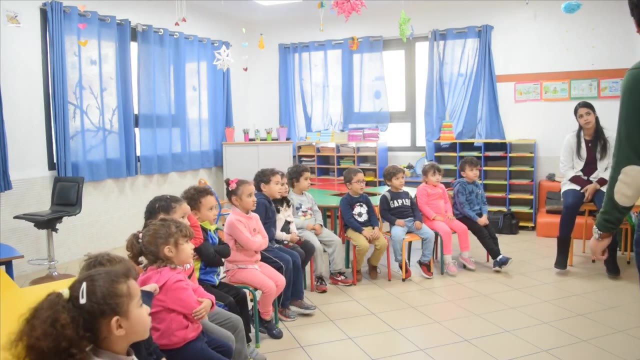 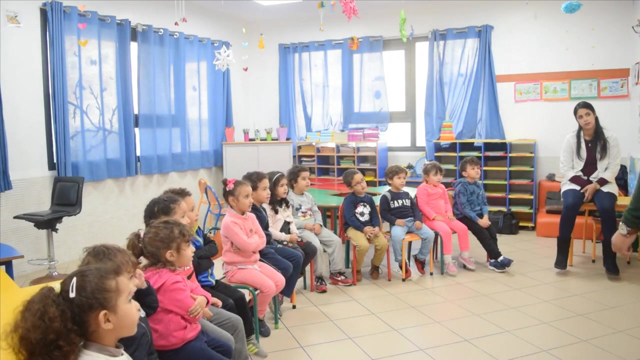 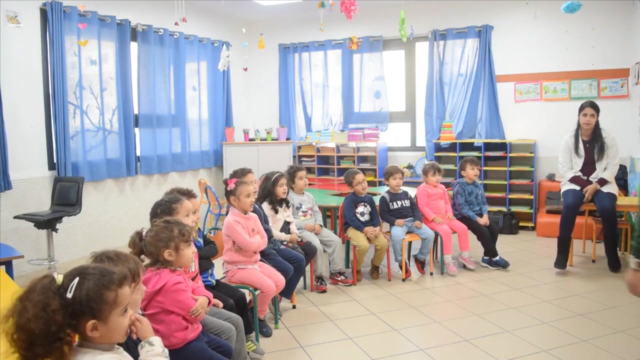 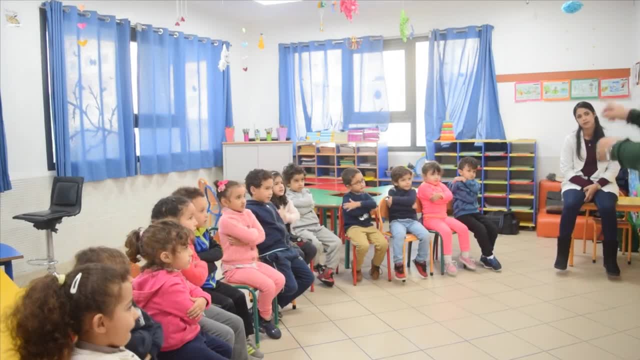 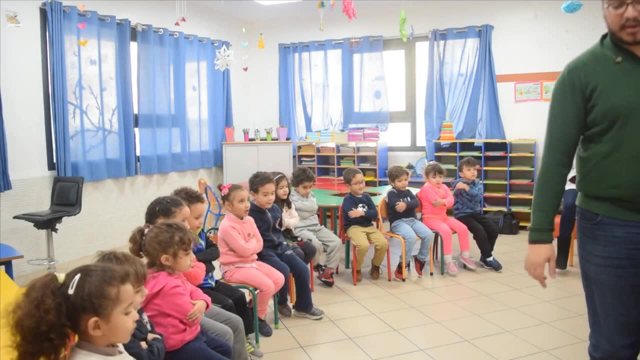 Now, look, we're going to play a game. Let me see which game You're going to play with me. This game is like this. Here we go. Here we go: 1, 2,, 3,, 4,, 5,, 6,, 7,, 8,, 9,, 10.. 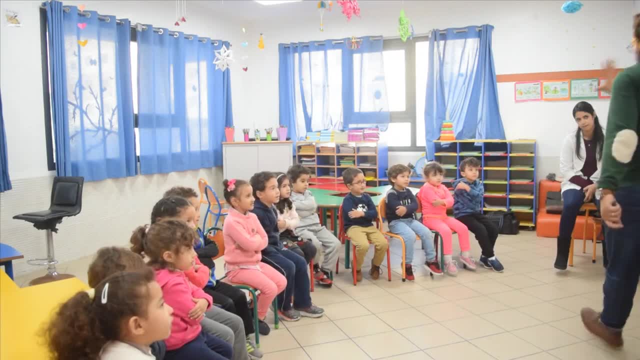 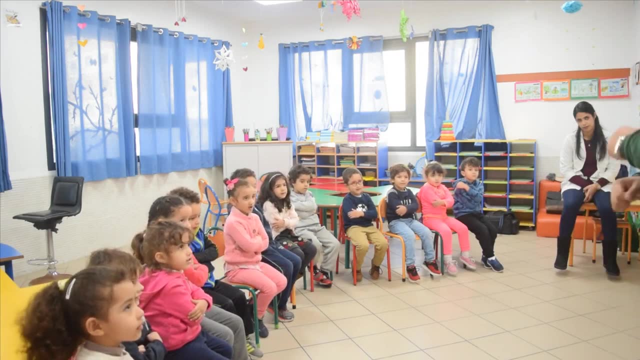 Jump. But you know we're going to do it just with 5.. Let's start with 5.. 1,, 2,, 3,, 4, 5. Jump: 1,, 2,, 3,, 4, 5.. 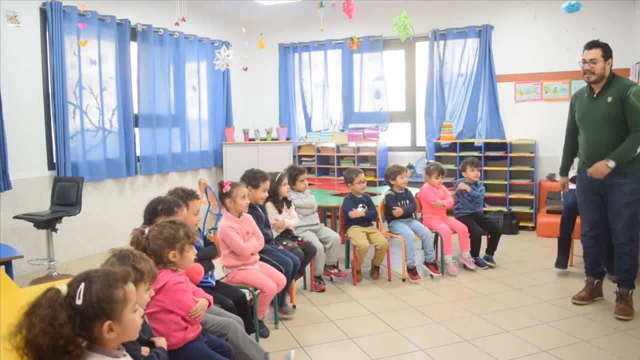 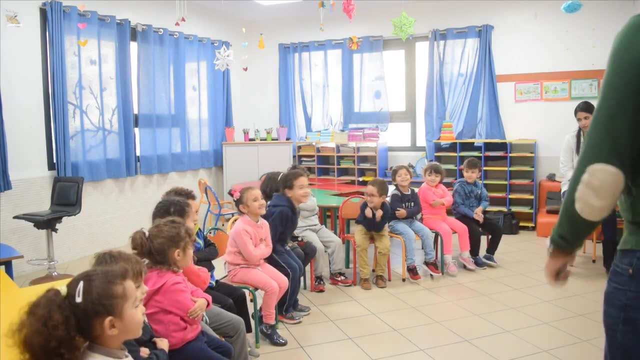 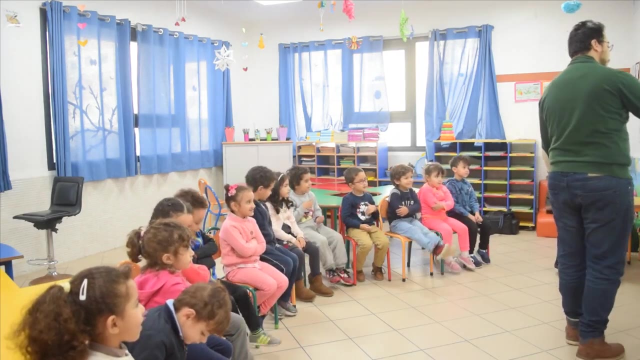 Kick, Kick, 1.. 1,, 2,, 3,, 4, 5.. Wiggle, wiggle, wiggle. Can we do it? Let's do it with some music here, right Music? Where is my music? It's right here. 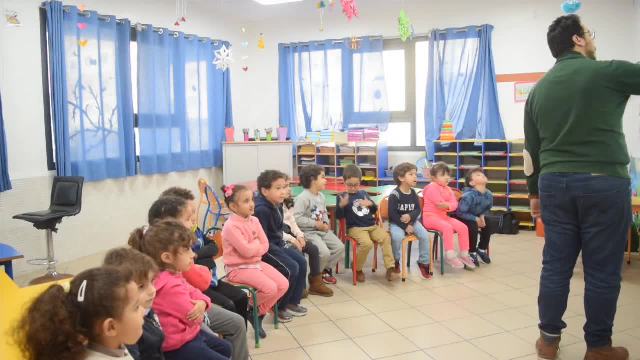 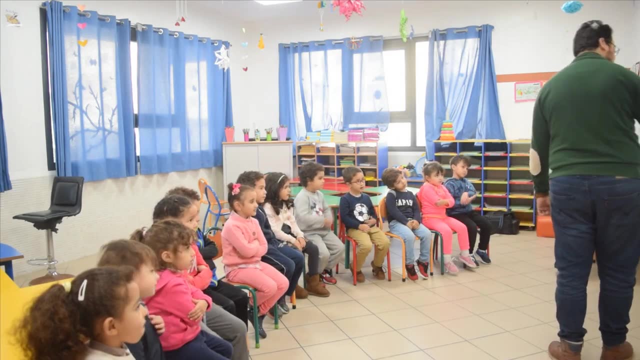 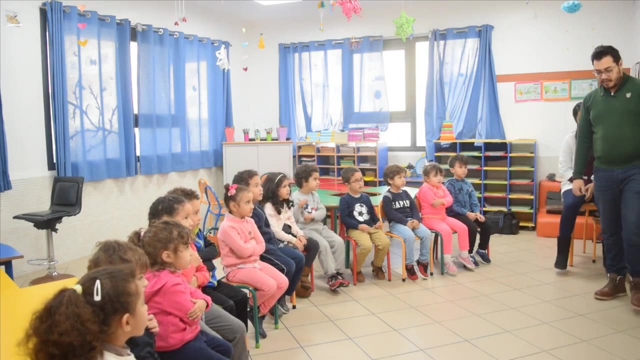 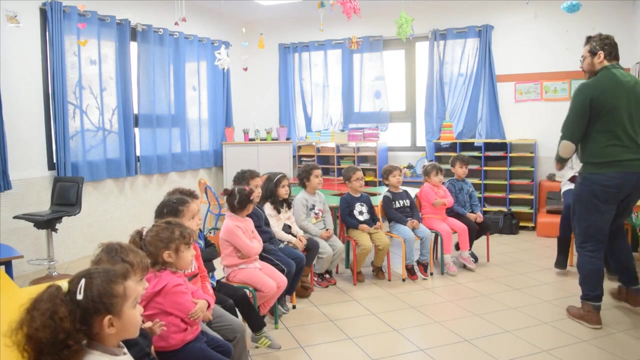 And where is my California song? It's right here too. Okay, so it's going to be like this: Let's take a slip: 1,, 2,, 3,, 4, 5.. Jump 1,, 2,, 3,, 4,, 5.. 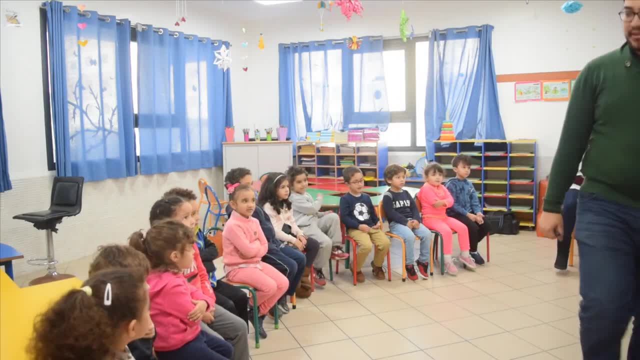 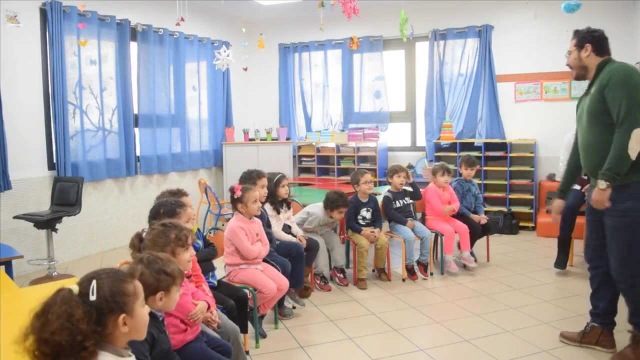 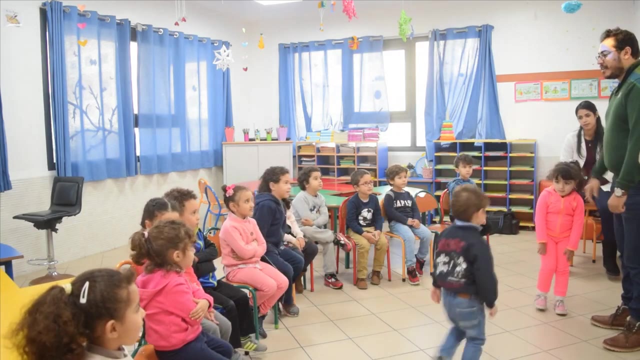 Kick, Kick, 1,, 2,, 3,, 4, 5.. Wiggle, wiggle, wiggle. Okay, Let's do it together. Come here Maria, Come here Maria And come here Jean. 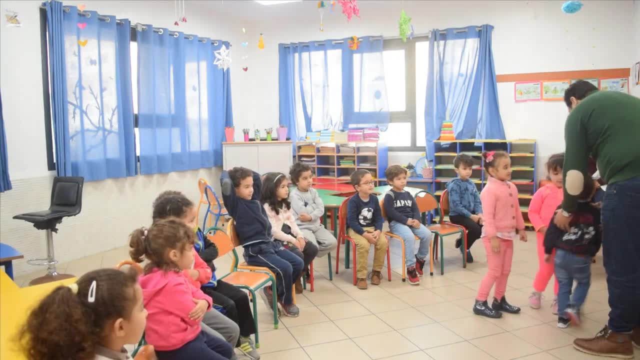 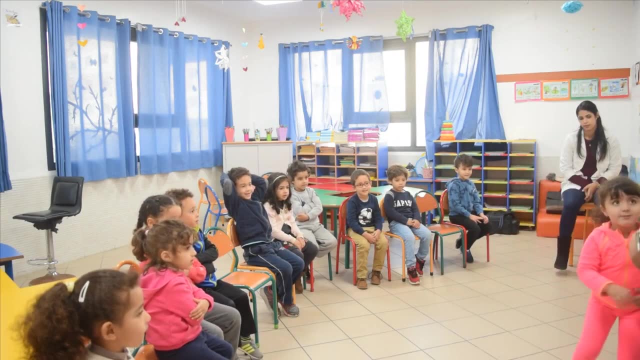 I already have my MGM. Okay, let's do it. Okay, 1,, 2,, 3,, 4, 5. Jump, Jump. 1, 2,, 3,, 4,, 5. Kick. 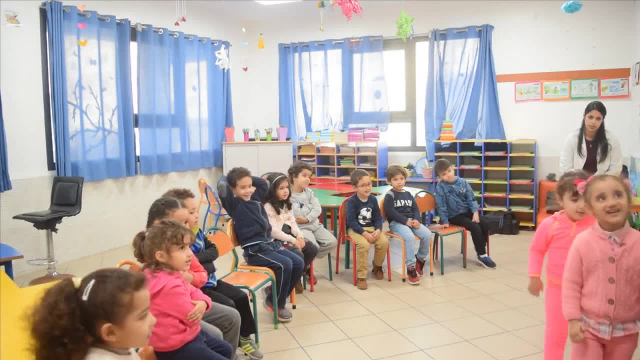 Kick, kick, kick. 1,, 2,, 3,, 4, 5.. Wiggle, wiggle, wiggle, Wiggle, wiggle, wiggle. All right, let's go Sit down Good. 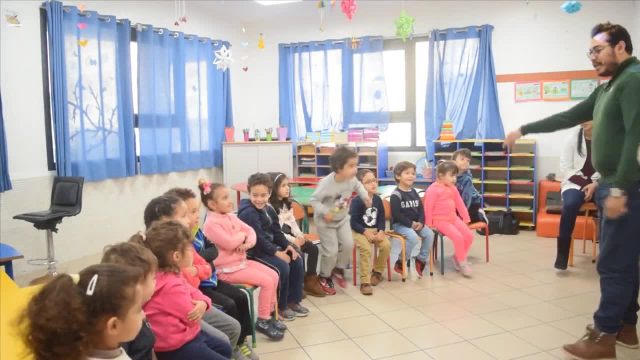 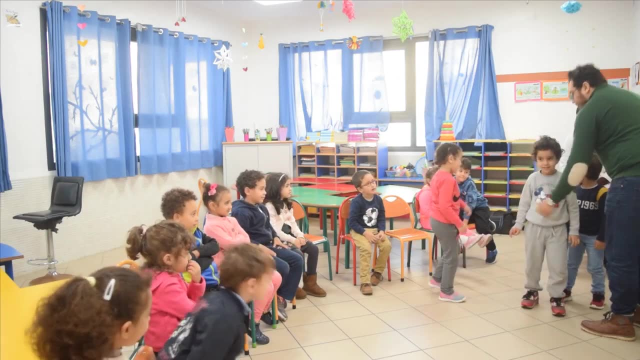 Let's take another three. We're going to take Adam Amin and DJ, And DJ, High-five, high-five. a little bit, Come back, All right, good, good, good, good, good. Okay, let's go. 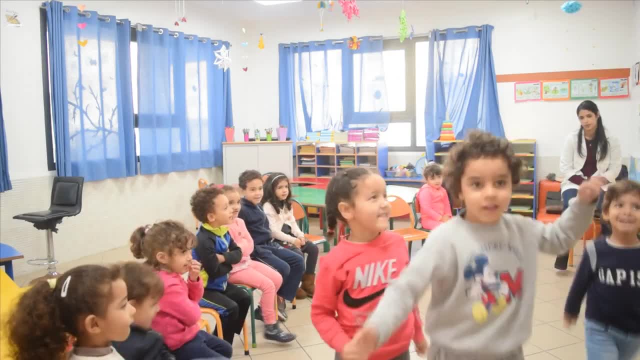 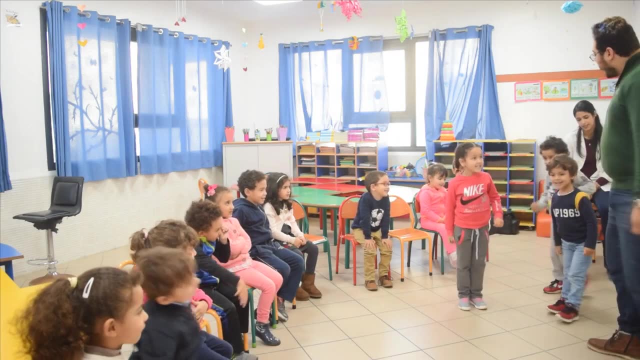 1,, 2,, 3,, 4, 5.. Jump, Jump 1,, 2,, 3,, 4, 5.. Jump, Kick, Kick 1,, 2,, 3,, 4, 5.. 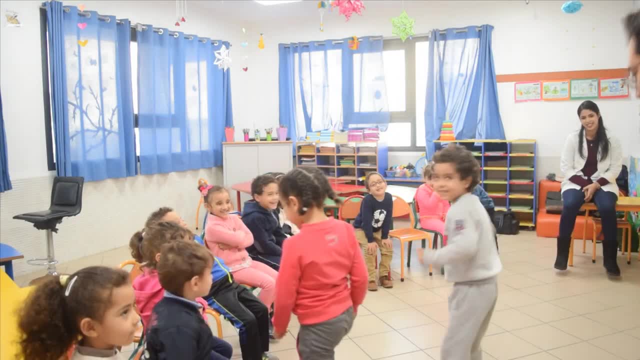 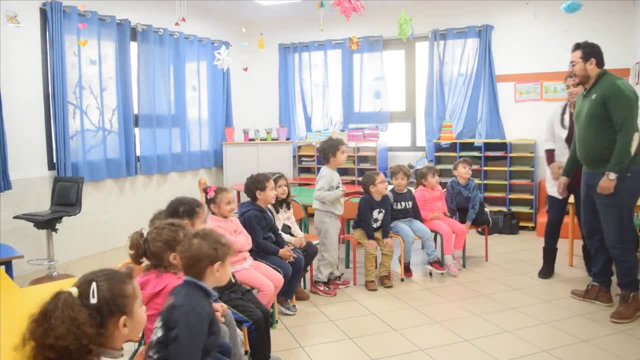 We're going to change. Okay, let's do it, Me and Karima and Jude. All right, Jude, come here. Yes, come here. Let's go 1,, 2,, 3,, 4,, 5.. 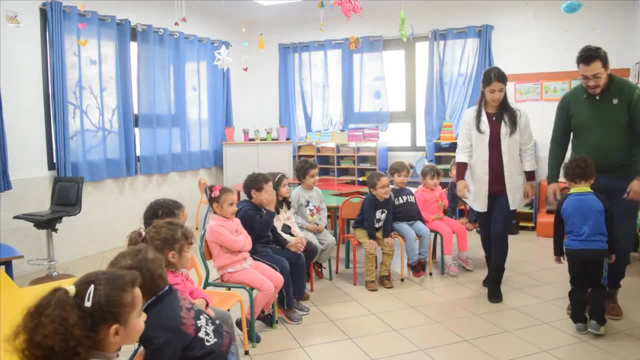 Jump 1,, 2,, 3,, 4,, 5.. Kick, Kick, Jude. kick 1,, 2,, 3,, 4,, 5.. Wiggle, wiggle, wiggle, Wiggle, wiggle, wiggle. 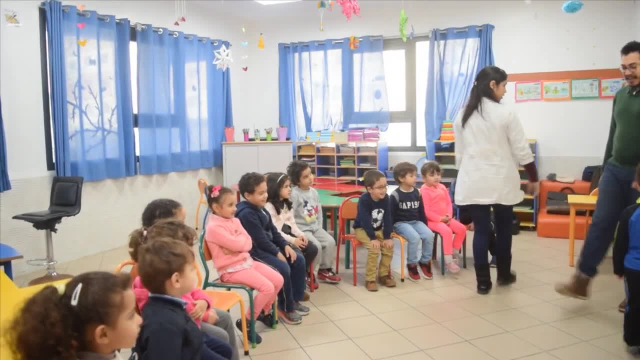